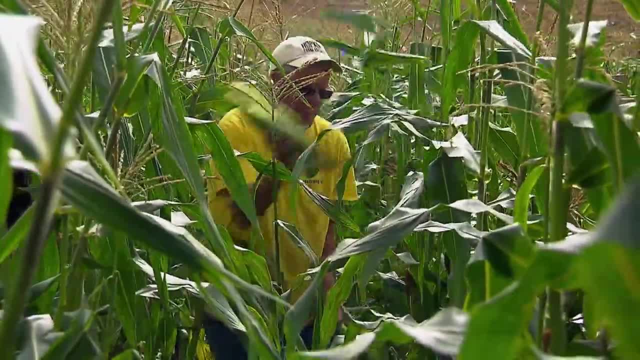 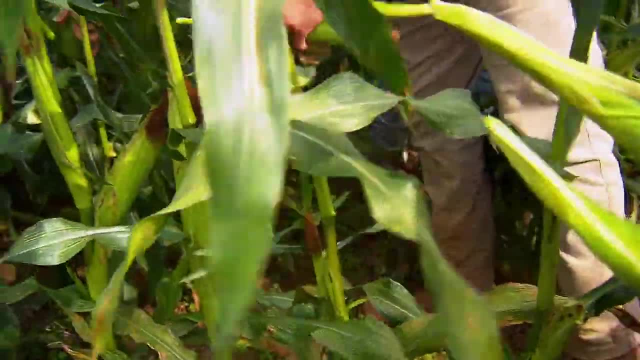 40 years on their 200-acre family farm in Haverdegrace. While sweet corn is their most popular crop, they raise a variety of produce. So we got the sweet corn, you know: tomatoes, strawberries, cantaloupes, watermelons. In addition to that, we got field corn, suey beans. 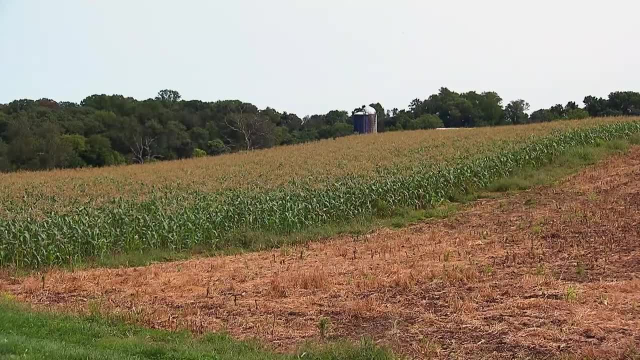 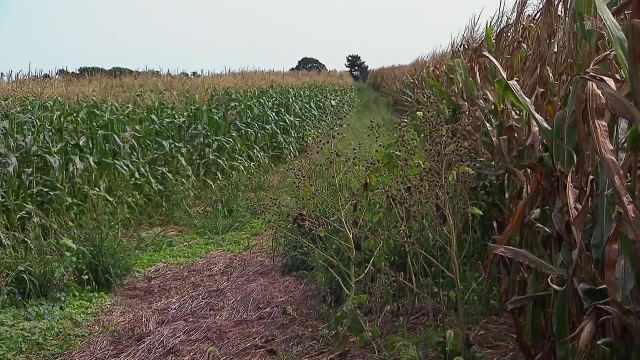 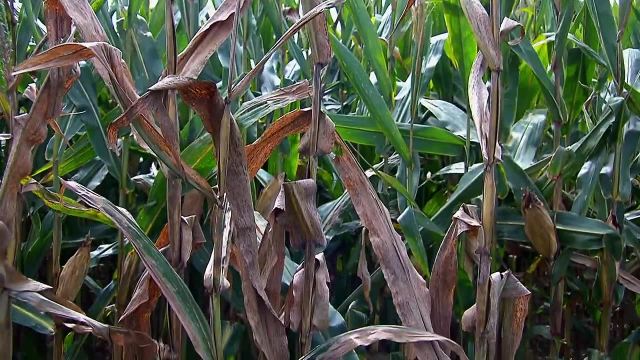 barley a little bit of hay. The biggest chunk of that would be sweet corn, which is about 30 acres. They might look the same to the untrained eye but compared to the sweet corn on the left, the field corn on the right is taller, thicker and sturdier. And the differences don't stop there. 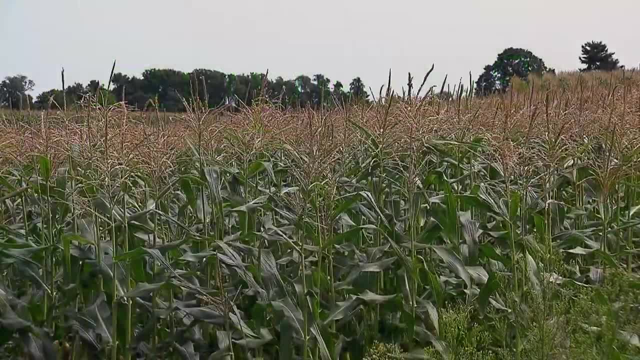 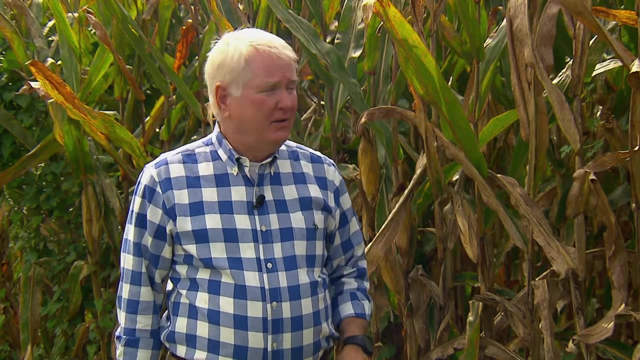 So you're driving down a country road and you see a beautiful green field of corn, but what you're looking at is sweet corn. It looks like this, all nice and white and tender. You go a little bit further and you see the corn looking like this, all dried out and brown and 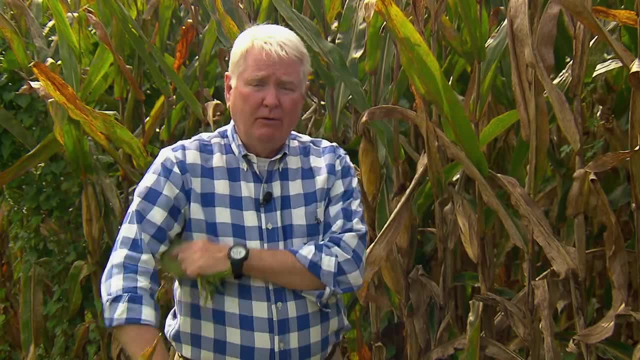 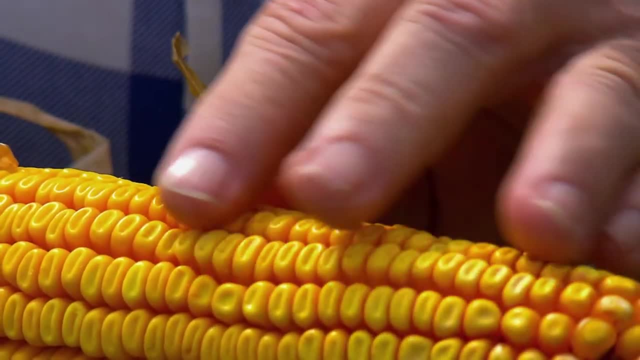 everything You think, my goodness, they're having a drought. No, what they're doing, they're growing field corn and it looks like this. They're leaving the cobs out there to get nice and hard. so don't ever try to bite down on these, because you'll break your teeth. 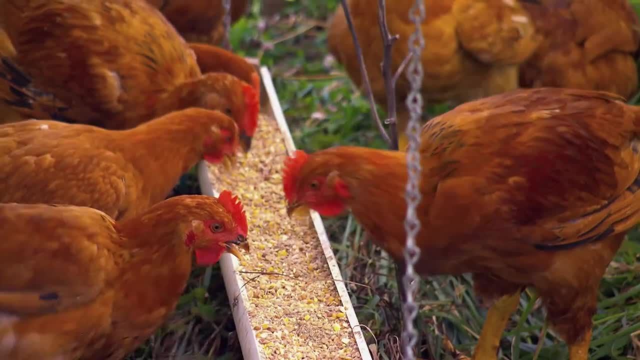 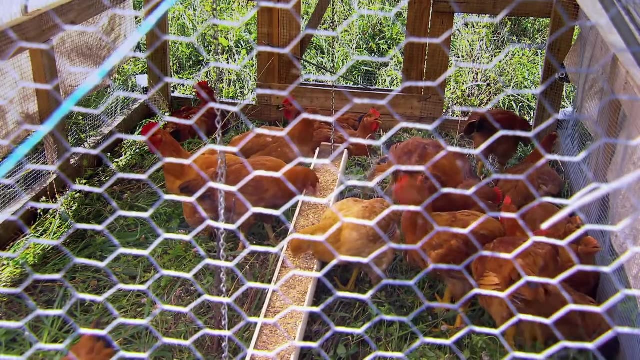 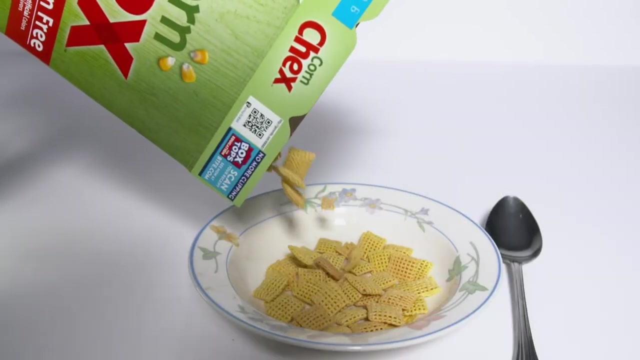 However, it's great for chickens, eggs and cows. That's because most field corn is intended for livestock feed, although some does make its way into your kitchen, just not necessarily on the cob. Field corn's processed. You got your cereal stuff to choose. for What else, you got Corn syrup. 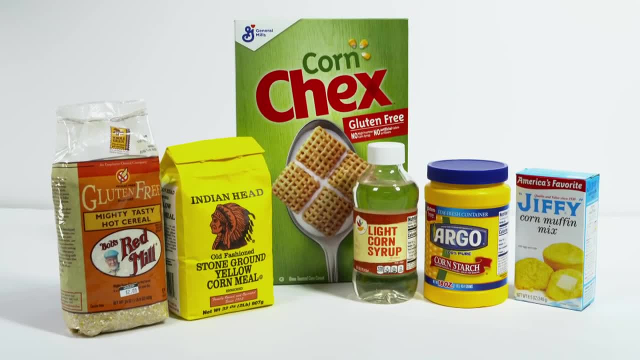 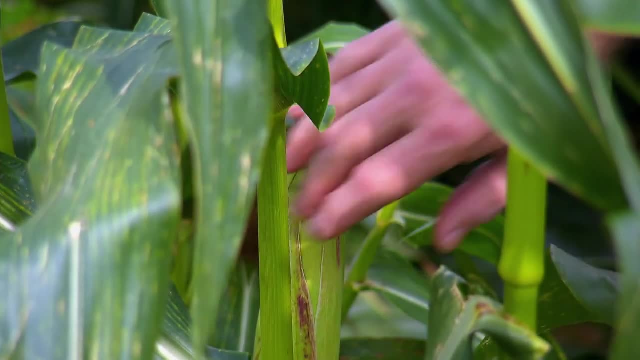 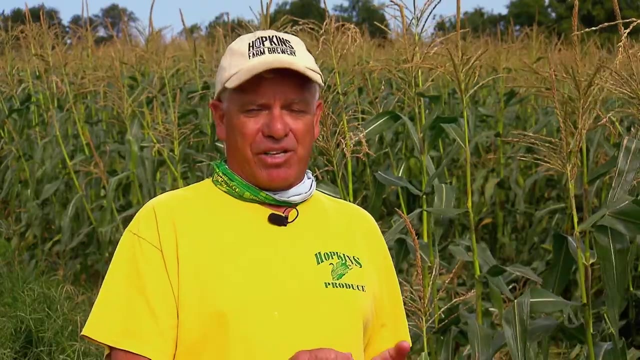 corn, starch corn, all kinds of corn products. While the Hopkins harvest their field corn by machine, for the sweet corn they prefer a human touch. There is a lot of sweet corn that's picked mechanically. There are bigger operations that have mechanical sweet corn pickers. It's still got to be sorted going through. 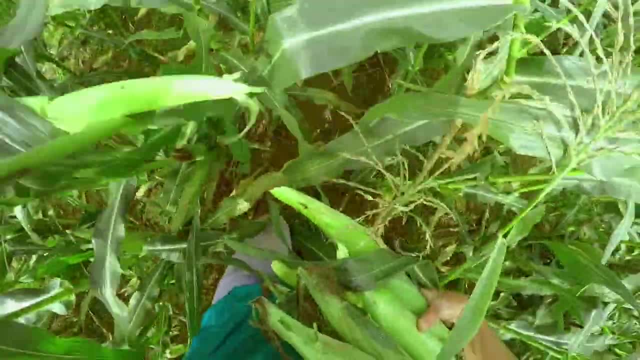 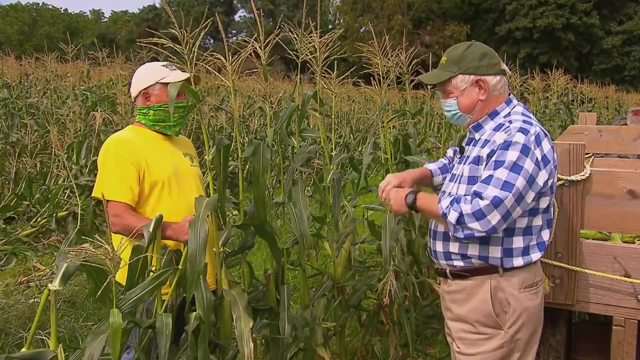 and a lot will be thrown out, and a lot of your sweet corn. it's just not all ready at the same time. Now I've noticed that when you go through actually picking there's a little bit of a technique involved. Can you show me I'm right-handed, but I pick corn left-handed anyway? 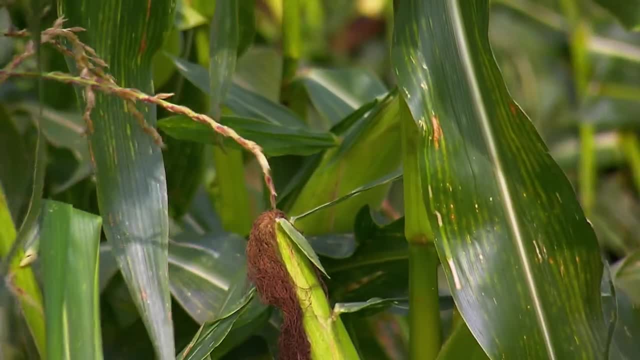 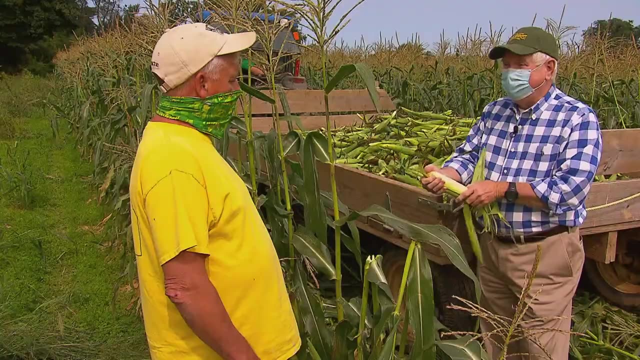 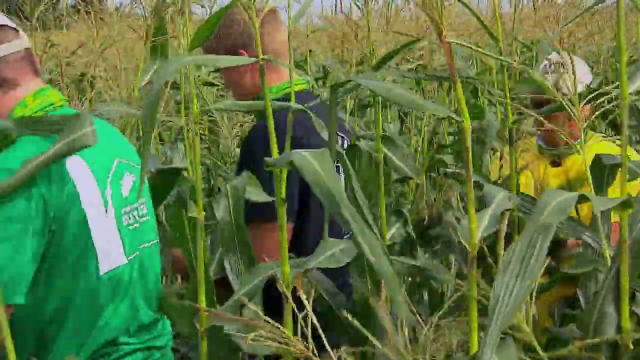 But anyway, I just kind of give it a twist on the snap and down. Well, Dave, let's see what this looks like in here. Oh my goodness, That's pretty, Looks good, That is really pretty, And Dave's favorite part of picking sweet corn.